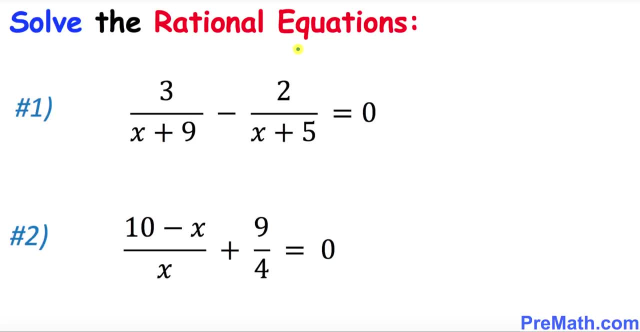 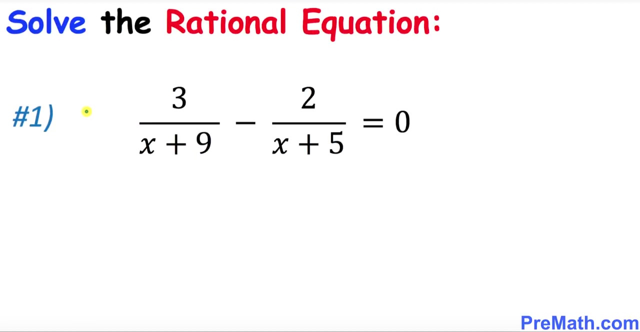 Hello again everyone. In this video tutorial, we are going to solve these two given rational equations And, by the way, these equations are called rational because we are simply dealing with these fractions. As you can see, these are just the fractions, So let's get started with the very first equation. So, always, whenever you have two, 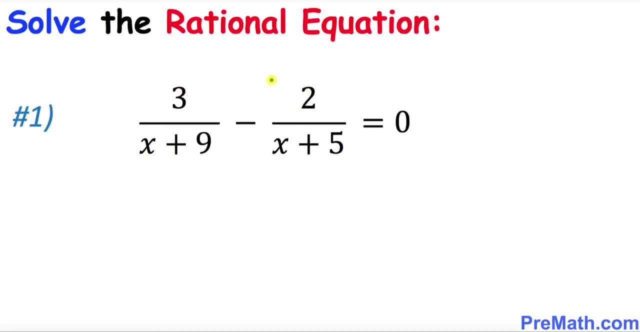 fractions and you have this kind of scenario always. do like this thing. I want you to move. drag this equation on the right hand side So this simply becomes 3 over x plus 9 equals to when you move this negative sign, and the other becomes simply 2 over x plus. 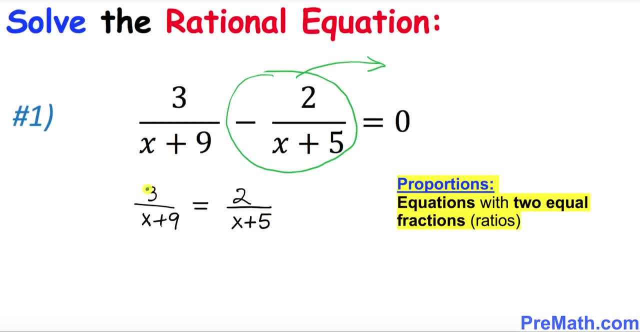 5. Now, as you can see, we have one fraction on the left hand side and the other fraction on the right and an equal sign in between. So this kind of scenario is called proportion. So these are called proportion. That means they have an equal sign in between these two. 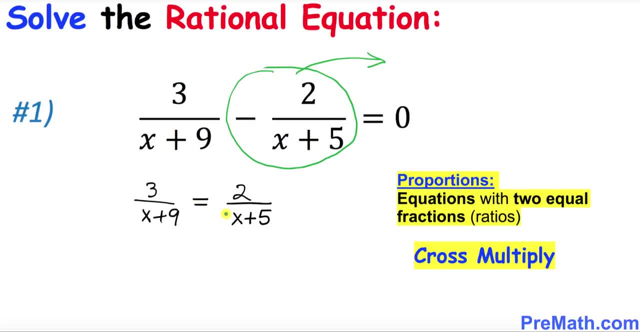 fractions. So we are going to solve this given equation by using a cross multiplication. That means we are going to crisscross, Multiply this way and multiply this way. So let's go ahead and multiply this 3 times x plus 5 and write it down over here. I'm going to 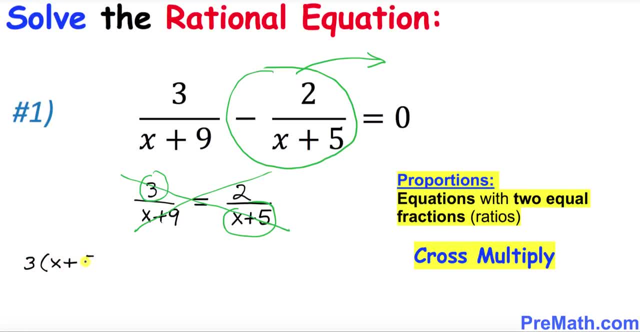 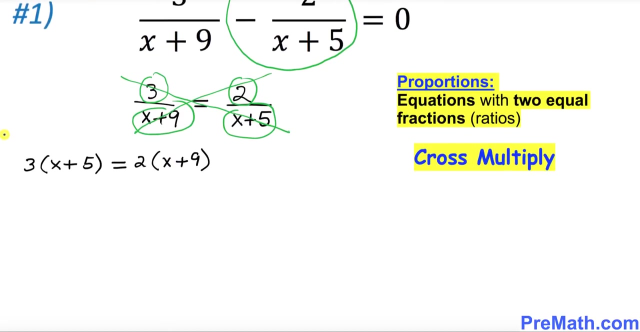 write down: 3 times x plus 5 equals to: on the other way around, multiply this 2 times x plus 9.. So I can write 2 times x. So far, so good. So let's go ahead and distribute over here. I'm going to multiply this 3 with. 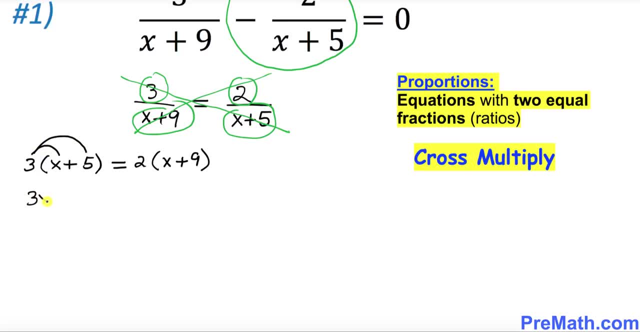 both of them. So this simply becomes 3x plus 3 times 5 is 15 equals to. likewise, we're going to multiply or distribute, So this is going to become 2x plus 18.. So I want you to subtract 2x from both sides, as you can see. So this 2x and 2x is gone, 2x minus. 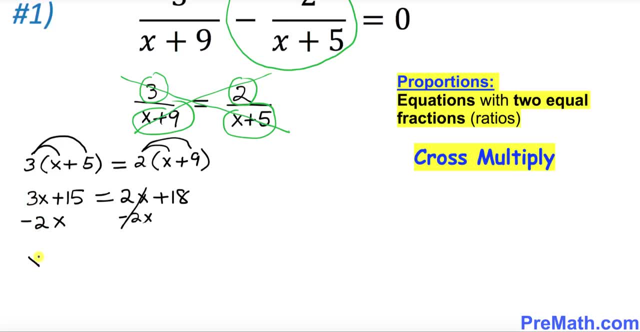 3x minus 2x is going to be simply 1x plus 15 equals to 18.. And I want you to subtract 15 from both sides, so x turns out to be simply 3, which is our solve problem solution. so thus our solution set turns out to be simply x equal to 3, and that is our answer. 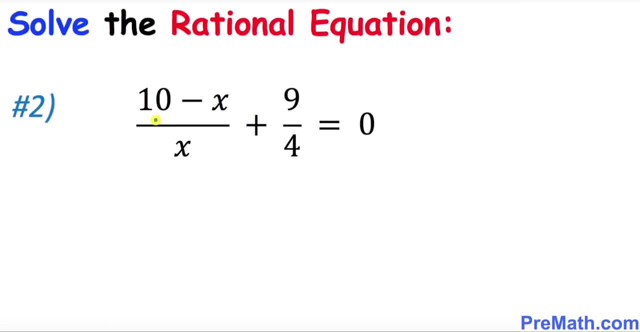 now we are going to solve this, another rational equation once again. the very first step is: i want you to let's do the simple way. i want you to look at this fraction, positive 9 over 4. i want you to move it on the right hand side, so this is simply is going to become x, 10 minus x divided by x. 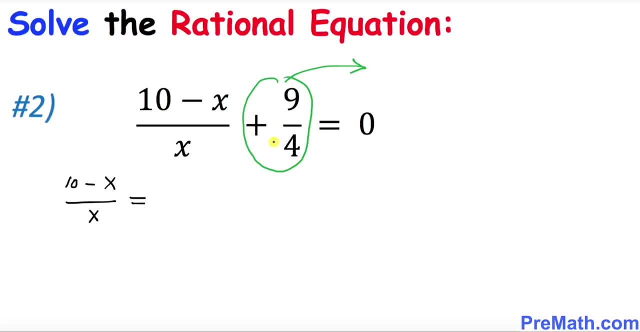 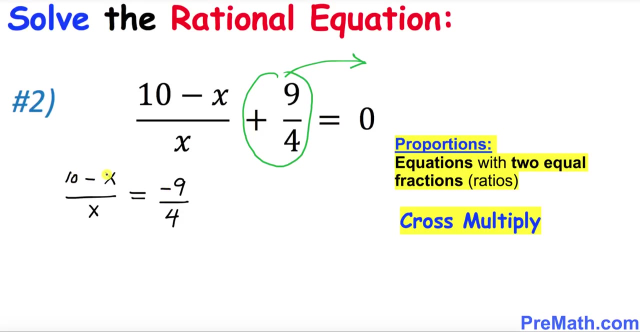 equals to when you move this positive 9 over 4 on the other side become negative 9 over 4, as you can see, and once again, this equation is just simply a proportion, as you can see, since we have two ratios, are two fractions and equal sign in between them. so we 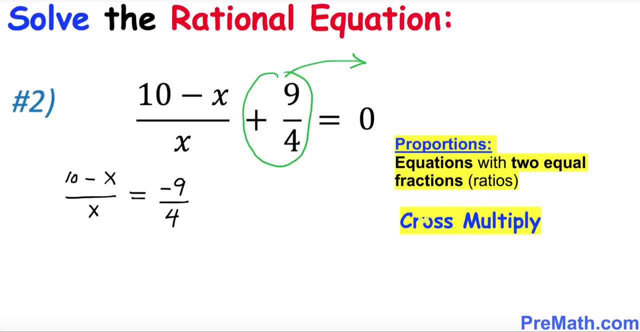 are going to solve them by using this cross multiplication method. so let's go ahead and cross multiply this way, we're going to cross multiply this way, and we're going to cross multiply this way. so if we cross multiply this way, going to be multiplying this 4 times 10 minus x, so let's go ahead and put it down: 4 times 10 minus x. 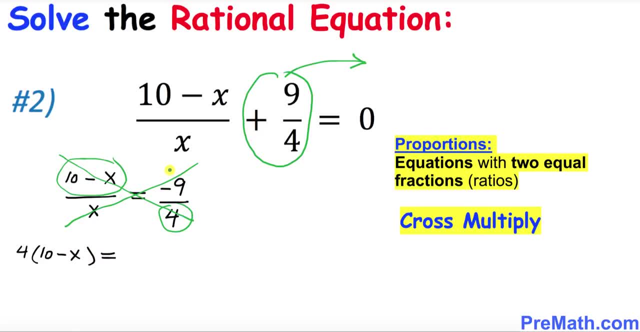 equals to. let's multiply the other way around: negative 9 times x becomes simply negative 9 x. so i'm going to write down negative 9 x. so the next step is: i want you to distribute right up here. so when you multiply, this become 10 times 4 is 40 minus 4 x, equal to simply negative.